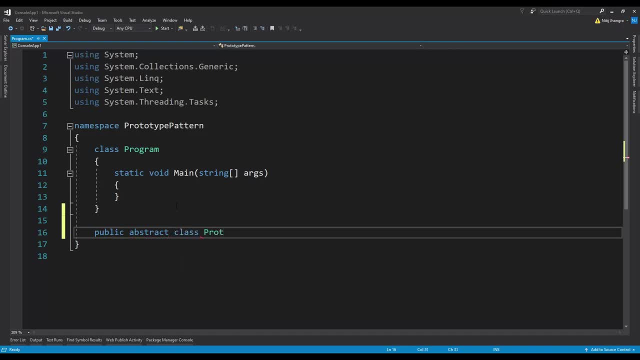 class or public abstract class and then prototype. So we will define the clone method. so public abstract prototype and then clone. Next we can create a concrete class that will derive from this prototype abstract class and it will implement the clone method. So this class can be for a 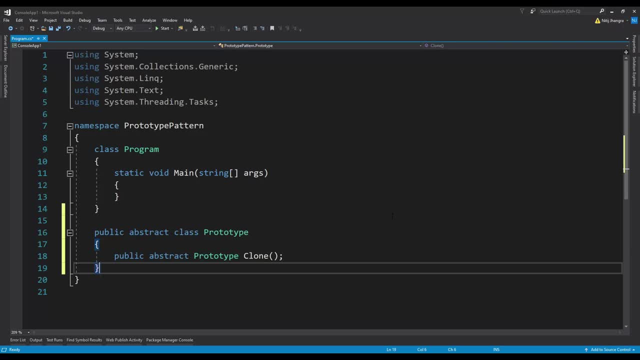 card. So if object is Seit, work can be for a custom class name. example: class is Isabelle, So that will also make a new class and saved it to our current object. Now, in order to control a and it may have properties like make, model year and so on. it might also have 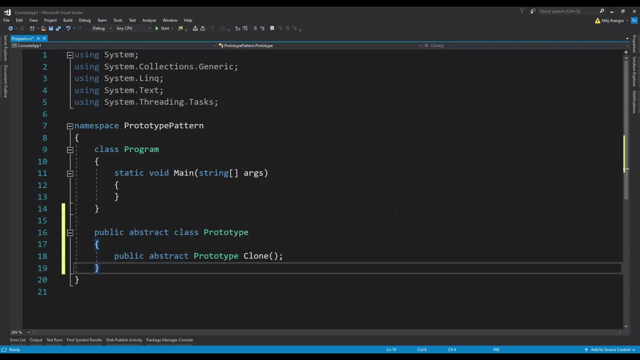 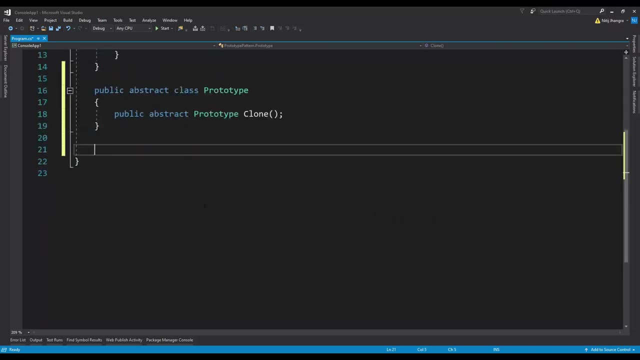 a constructor that will allow you to create a new car object with specific values for these properties. here is how this class can look like: so public class, car and then prototype. so let's add a bunch of properties, so public string, and then make- let's make- this an auto property. so let's add three more. so this: 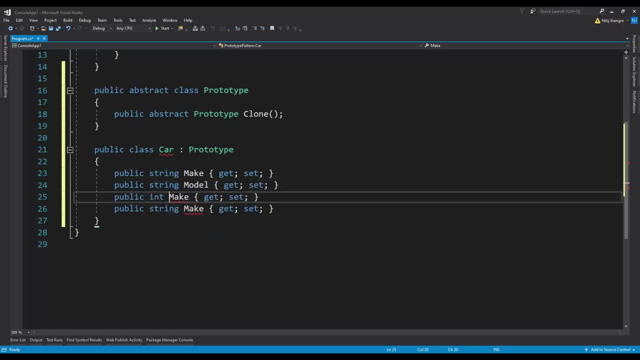 is going to be the model, this is going to be the year, and this is going to be a list of other options that this class will be using, so let's add three. more can have. so options. now. let's create a constructor, so public car, and then I'm. 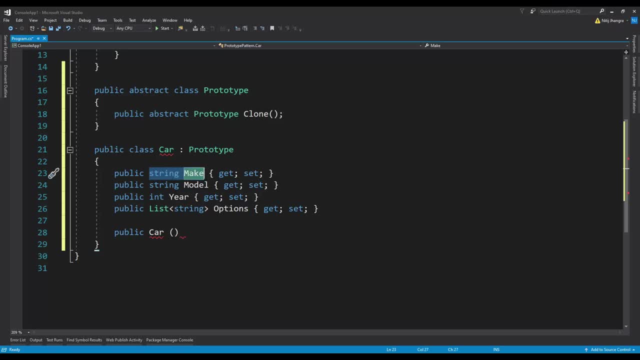 going to add all of these properties as arguments. so public car and then string make string, model, and then the eai and then the list of options. So make equals to make, and then model equals to the value of the model. argument here is here, and then options equals to options. 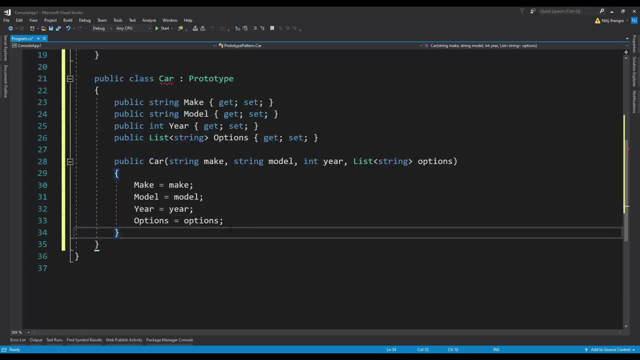 So now we have the constructor, It's time to provide the implementation for the clone method of the prototype class from which this car class is deriving. So public override and then prototype. It has automatically added the statement to throw a new, not implemented exception. but 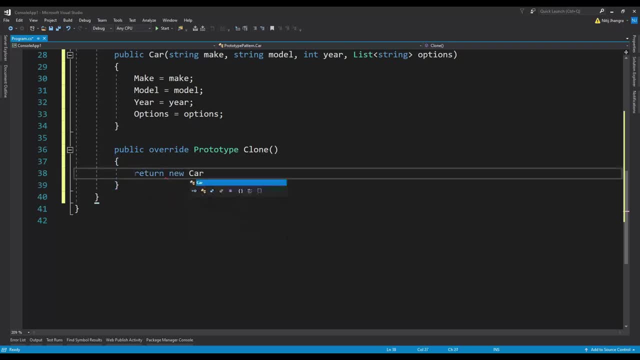 we are going to return a new car object with the properties which have been already set, So make model here, and then, instead of passing the options directly, we have to create a new list So that we will not be passing the reference of the existing list. 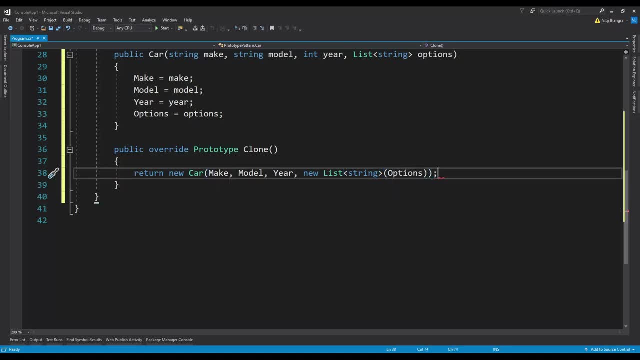 So we will provide the existing options list as an argument, And that's pretty much it. So, as you can see, this car class has the clone method, which creates a new car object with the same properties. Now that we have our prototype and car classes set up, we can use them to create new objects. 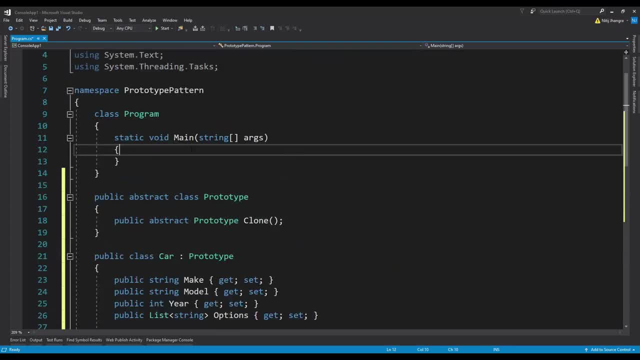 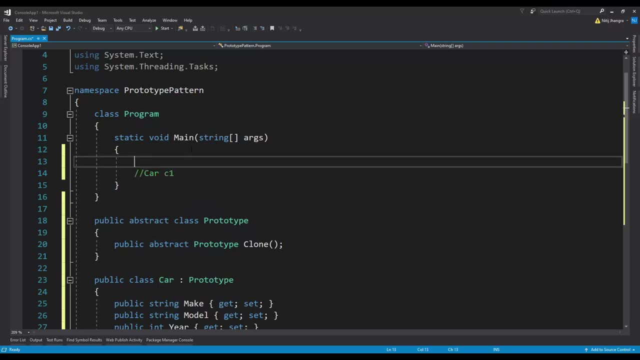 by calling the clone method on an existing object. So, for example, we can create a new car object. Let's create a new car object called as C1. But before that let's initialize the cars option object. So list of string options equals to new list of a string. and then let's provide a bunch. 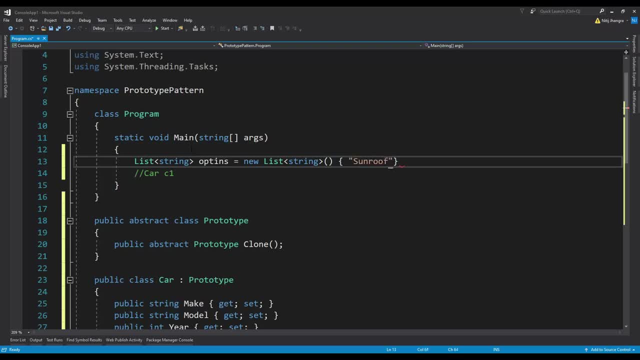 of options. So this car can have a sunroof, It can also have the navigation screen and it can also have, let's say, leather seats. All right, now for this C1 object, we can create a new car for the um, for the make. 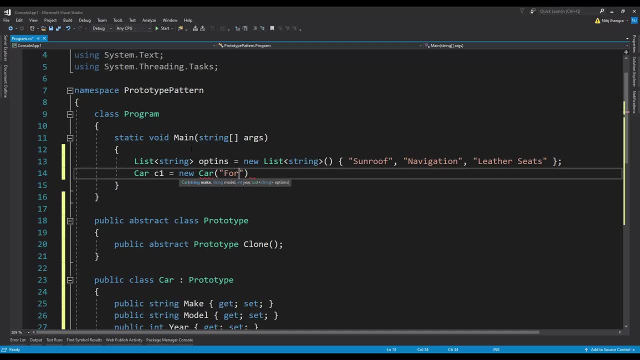 we can provide the brand name, which is Ford. model is Mustang. for year, I'm going to provide 2020, or you know what? let's use 2022 and then we will provide options. Now here is a red line. It is because I have misspelled this options. 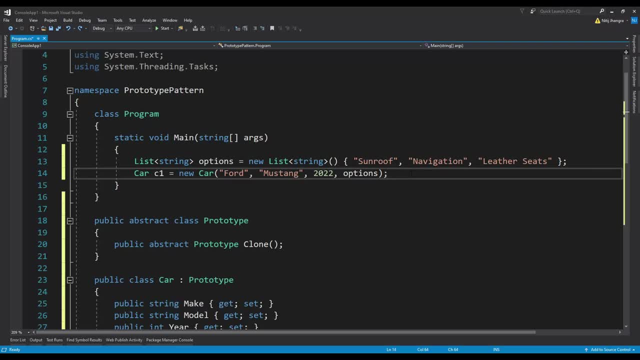 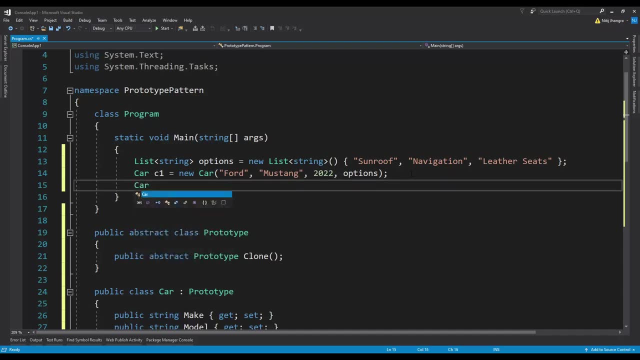 So we have this C1 car object and we can use the clone method to clone this existing object to create a new car object. So let's do that. car C2 equals to C1 dot loan And we also have to cast it as a car type and, as a result of cloning it, C2 will be.